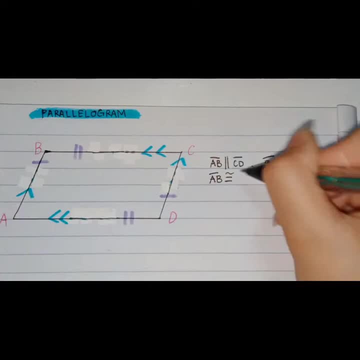 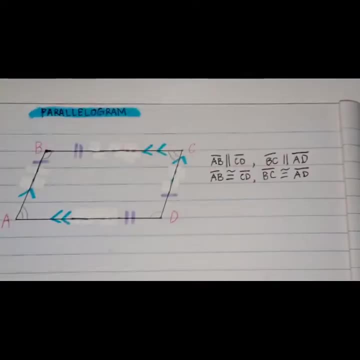 sides are congruent. That means A- B is congruent to C- D and also B- C is congruent to A- D. Opposite angles are also congruent, So angle B and angle D are congruent to each other. 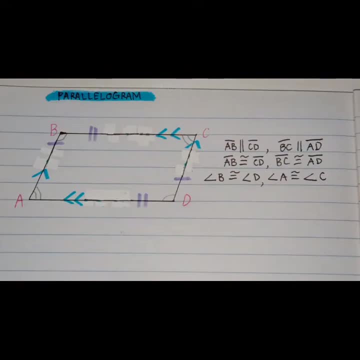 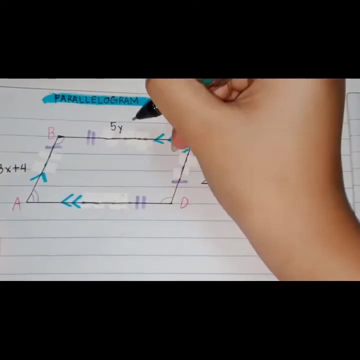 And also angle A is congruent to angle C. So now let's have our problem. Let's say: A- B is equal to 3x plus 4. B, C is 5y plus 3. C- D is 7x. 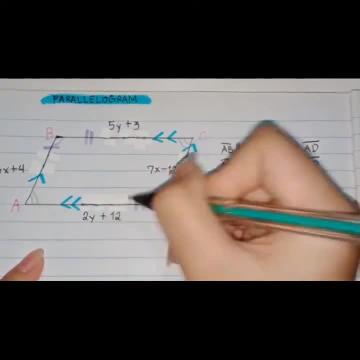 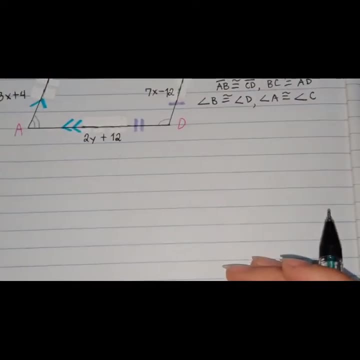 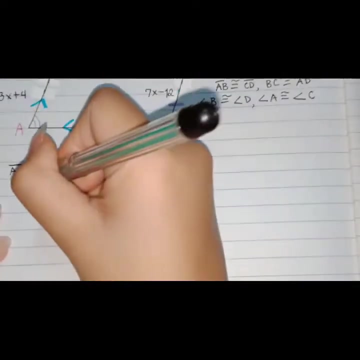 Minus 12 and 2y plus 12 for A, D. So with this information let's now solve our unknown variables. So first let's find the value of x. So let's write: A B equals C, D, 3x plus 4 equals. 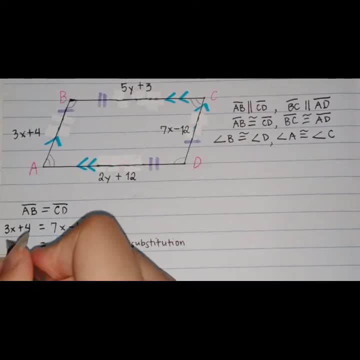 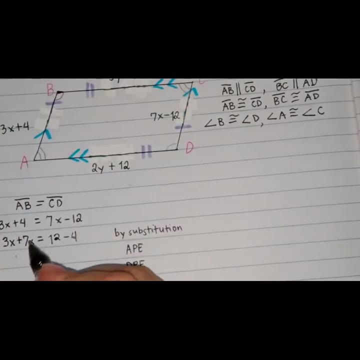 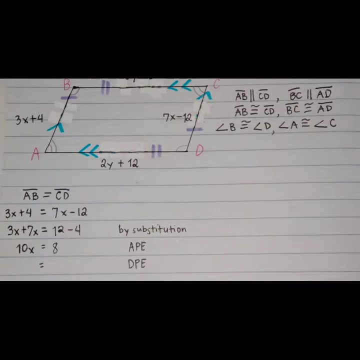 7x minus 12.. Due to transportation, now we have 3x plus 7x and 12 minus 4.. Using the addition property of equality, now we have 10x and 12 minus 4 is 8.. To find the: 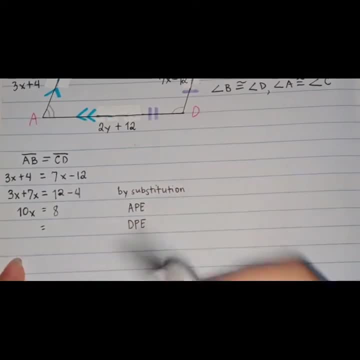 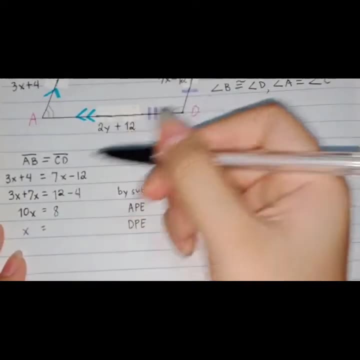 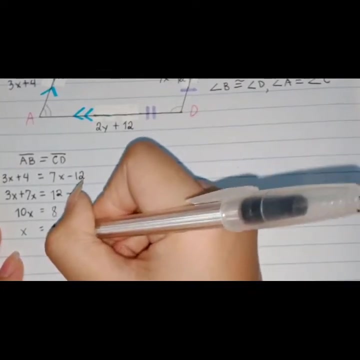 value of x. we're going to divide this both sides in, So 10 divided by 8 is really 1 times 25, but it's still 1. so let's make it 1 or just x, And 8 divided by itself is 1.. Now let's 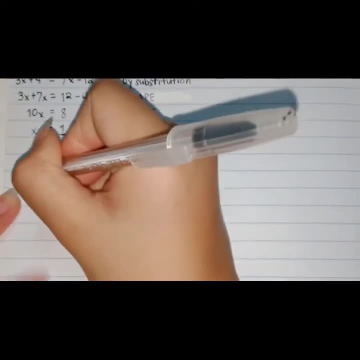 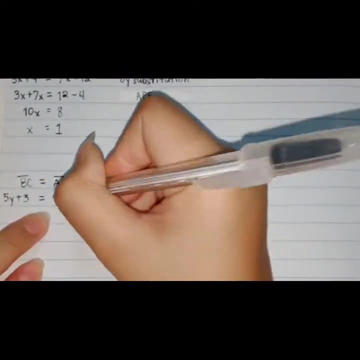 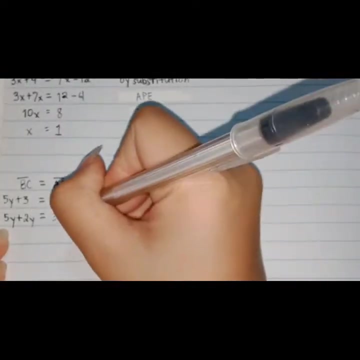 move on. So we have B. C is congruent to A, D By substitution. we transport this 2y beside the 5y and 3 beside the 12.. As usual, we're going to use the addition property of equality. 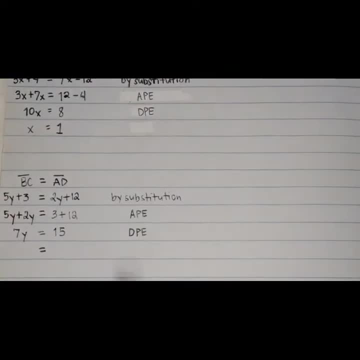 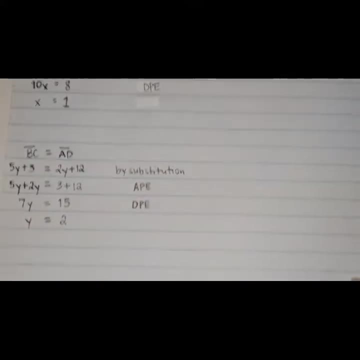 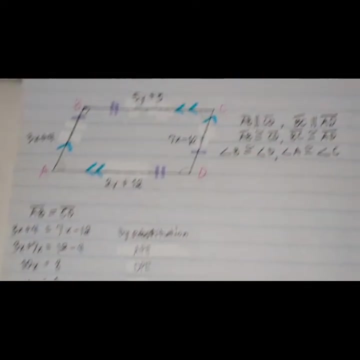 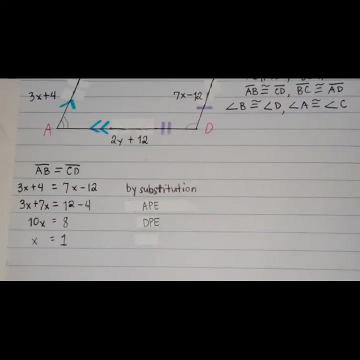 to sum it up, And lastly, we use the division property of equality to get the value of y. Therefore, the value of x is 1 and y is 2.. And that's it. It may be a little hard and confusing at first, but as you learn it, it would be so easy for you.